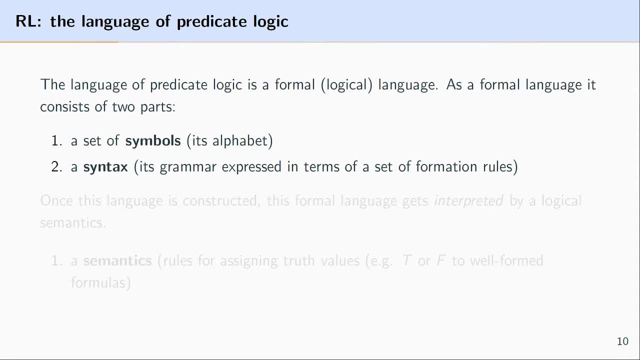 of a set of symbols and a syntax. The symbols are simply its base notation, or alphabet if you will- and the syntax: all it does is express the appropriate or grammatical way of putting those symbols together. So you have a host of symbols and specialized notation, and that's a. 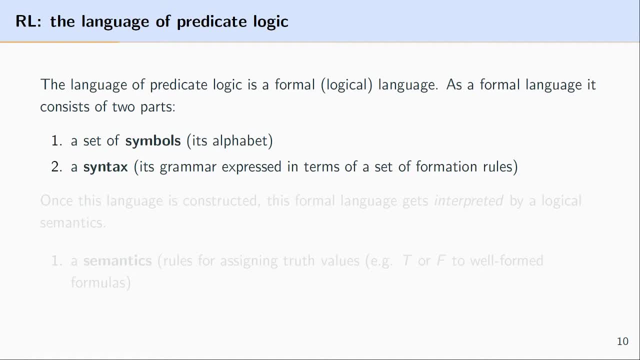 set of symbols and the syntax says: here's the proper way you can put those symbols together, and that's what a formal, logical language is. But there's always another aspect of a logical language and that's its semantics. Once you have this formal, logical language, you can put those symbols together, and that's what a formal, logical 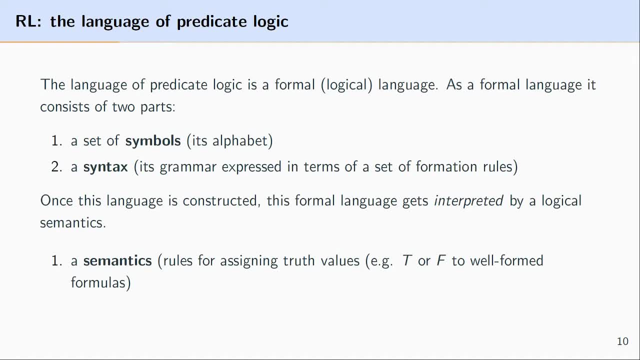 language. Then you say: okay, now, what does this language mean, What do these symbols mean and how do they get their meaning in combination with each other? That's what semantics essentially does. It takes those well-formed formulas those are, you know, might say grammatical sentences of the 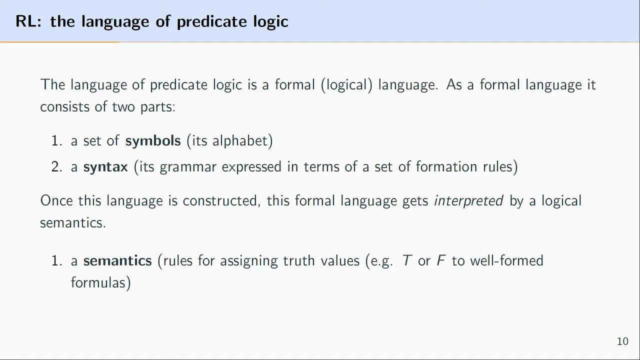 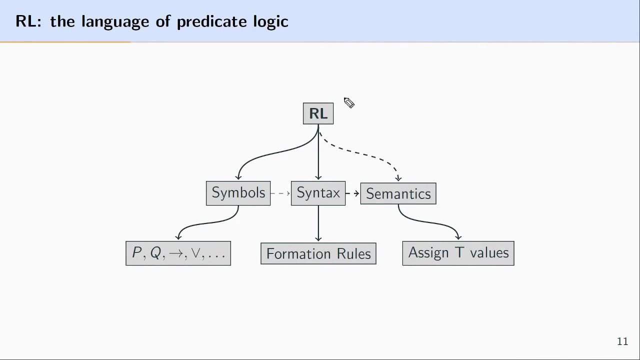 language and then it will use different functions or features to assign them a truth value, Typically true or false. but there are other logical languages that have a semantics that you know does different things with them. So it's helpful to see our kind of visual diagram of this. So we have 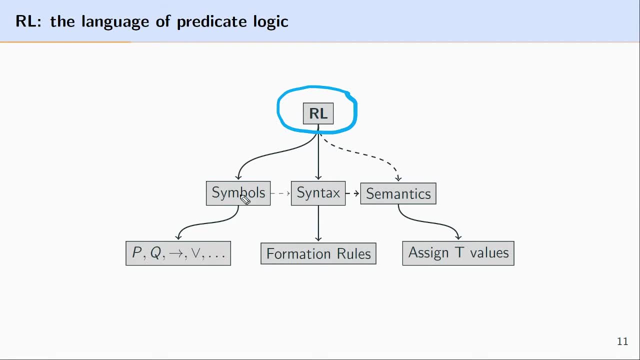 the logical language here, the language of predicate logic, and it consists of symbols. These are all the different letters that make up the language, and that logical language also consists of a syntax in terms of a set of like grammatical rules, and that's what the formal language is. It's just the 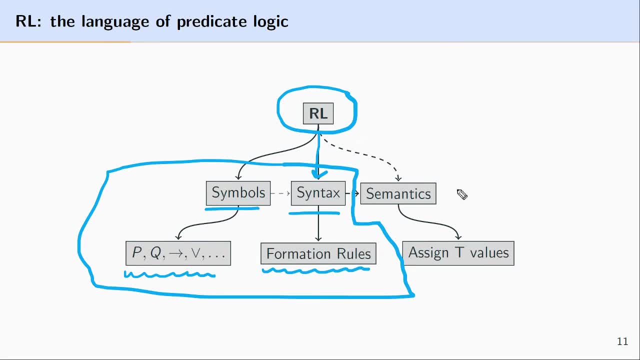 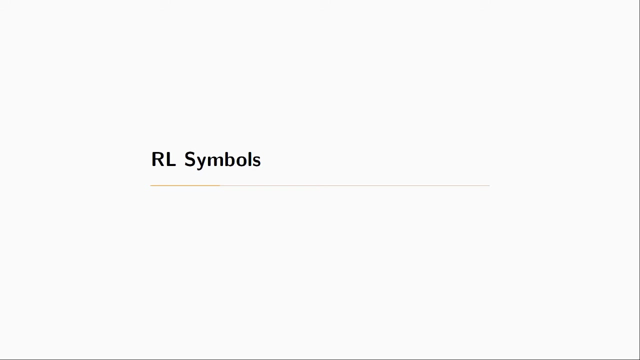 symbols and the syntax. Once we have this formal language in place, we'll go ahead and use various functions or rules to assign the well-formed formulas, the full units of the language, a truth value in terms of true or false. So, in the remainder of this video, what I'd like to do is talk about the symbols of predicate logic. 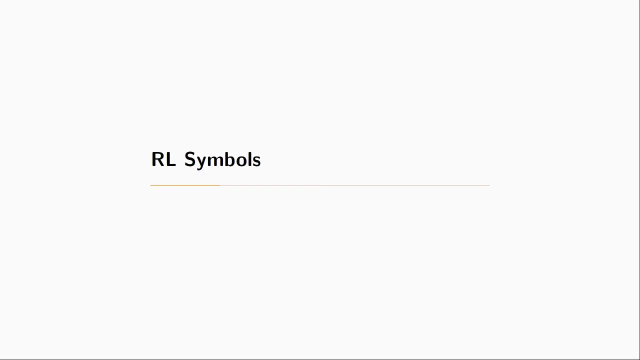 Here we won't talk about what the symbols mean, nor how to put those symbols together in a grammatically correct way. Instead, we'll just introduce the basic symbols, or alphabet, of the language. So the first set of symbols to look at are called names, and names refer to lowercase letters. 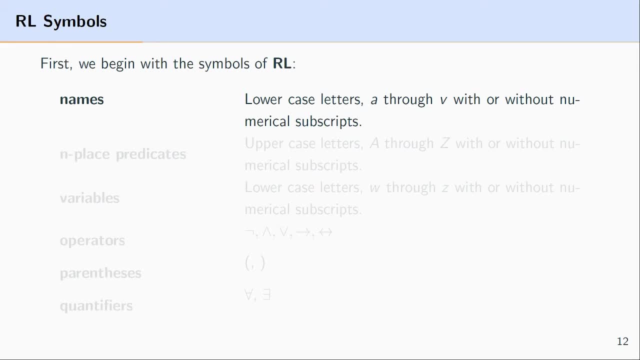 A through V, with or without numerical subscripts. So let's take a look at some examples here. So the letter A is the name, B is a name and C is a name. But since we don't want to be limited simply to the 23 or 24 letters right here, 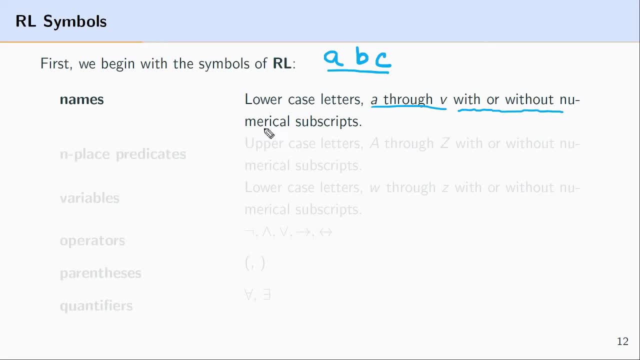 Instead we want an infinite number will allow for subscripting positive integers to these names. So A sub 1 will be a name, A sub 2 will be a name, A sub 3 will be a name, and so forth and so on. 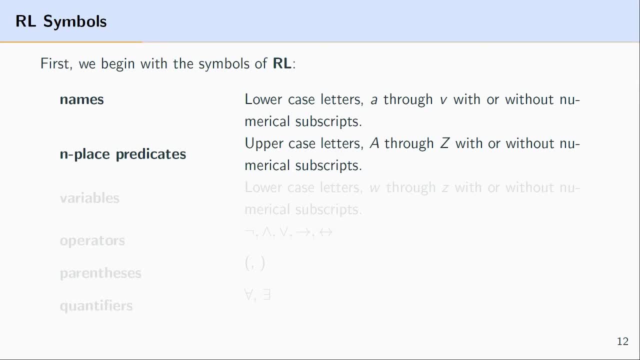 the next symbol that we look at are called end place predicates, and place predicates refer to uppercase letters A through Z, with or without numerical subscripts. So to look at a couple examples: A is an end place predicate, B is an end place predicate And C is an end place predicate, And we could kind of go on word and on word all the way to Z. 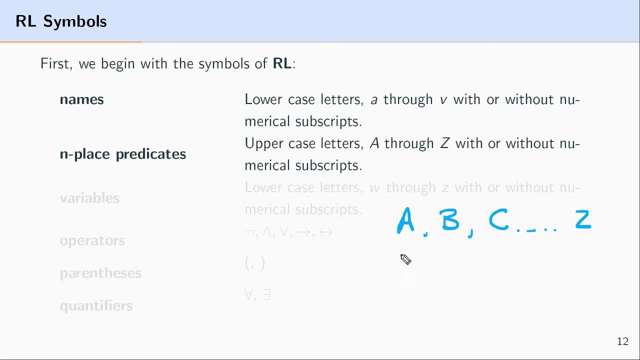 In addition, since we want an infinite number of end place predicates at our disposal will allow for A sub 1 to be an place predicate of end place predicates at our disposal will allow for a sub 1 to be a end place. predicate b sub 2 to be an end place. predicate c sub 50 to be an end place. 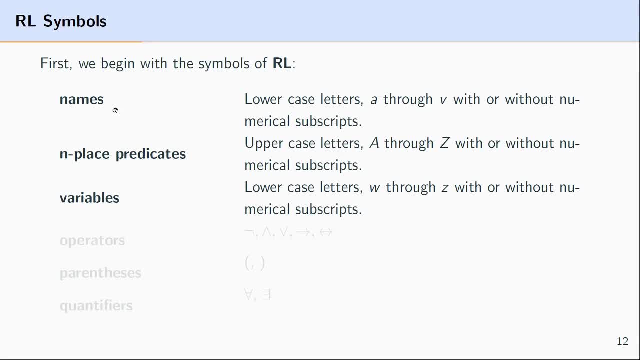 predicate, and so forth and so on. The next symbol to look at are called variables, and variables refer to lowercase letters, w through z, with or without numerical subscripts. So, for example, x will be a variable, y will be a variable, z will be a variable as well as w, And again, since we want an infinite, 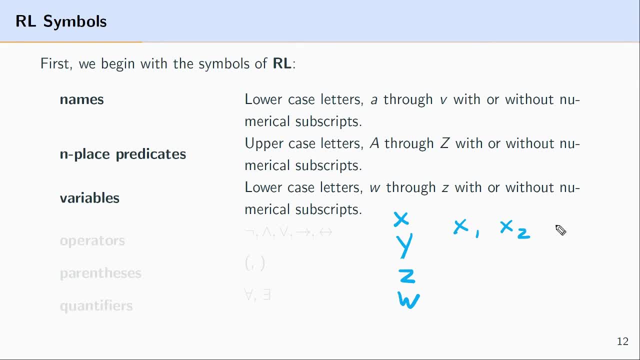 number, x sub 1, x sub 2, x sub 3 are all variables. In addition to variables, we'll have the truth: functional operators, sometimes shortened to just be referred to as operators. So we have the sign for negation, conjunction, disjunction. 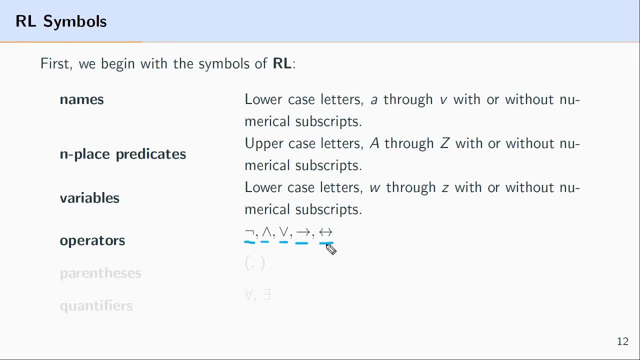 implication and the double arrow for biconditionality. So we have the sign for negation, conjunction, disjunction, implication and the double arrow for biconditionality. We'll make use of parentheses. In addition to parentheses, we'll